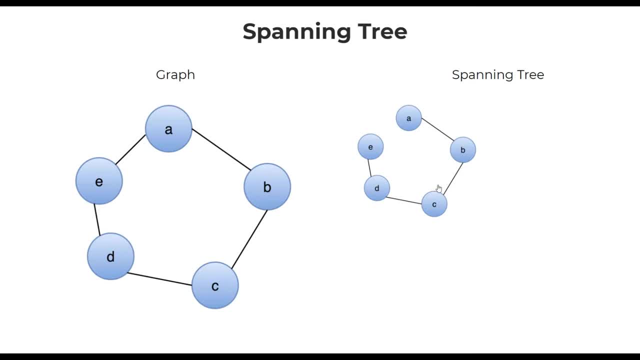 tree in which all the vertices are included. all the vertices are connected. we cannot leave a vertex like this that is disconnected from the rest of the vertices, so this cannot be a spanning tree. now, a graph can have more than one spanning trees. if you take this graph and ignore the edge. 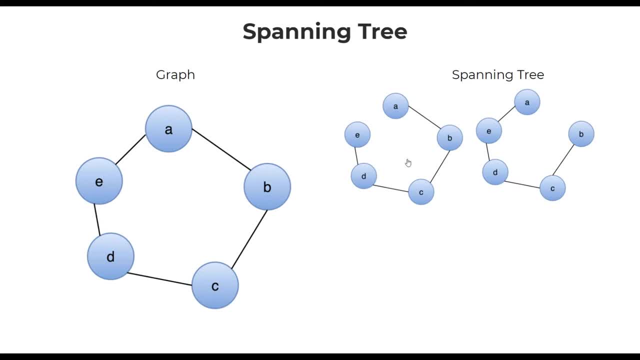 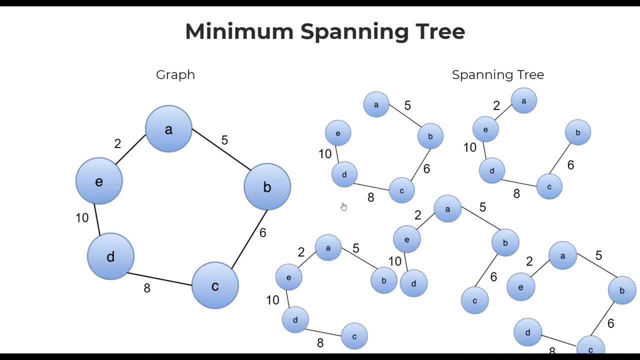 between a and e, then we get a spanning tree. if we ignore this edge, we get another spanning tree. similarly, we can construct three more spanning trees for the same graph. minimum spanning tree. the term minimum comes into picture only when we have weighted graphs like this for all these five. 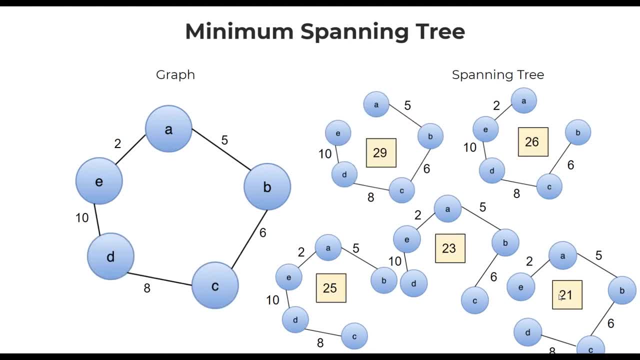 spanning trees. if we calculate the total cost, we get five different values. the one with the minimum total cost becomes the minimum spanning tree. minimum spanning trees are not necessarily unique. you can have more than one spanning tree. if we ignore this edge, we get another spanning tree, one minimum spanning tree for a given graph. why should we find minimum spanning tree? see here. 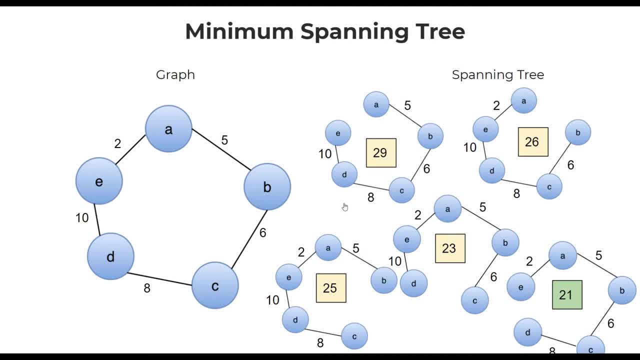 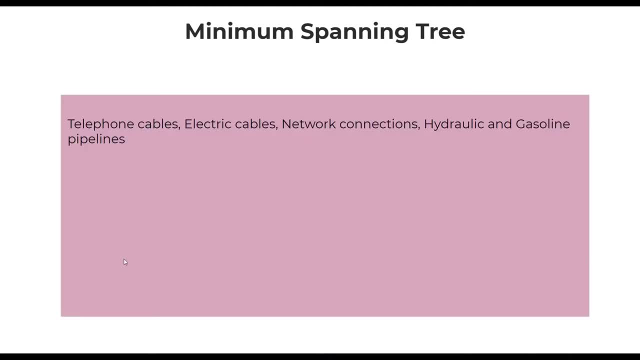 the vertices of the graph could represent different cities or different locations in a city, and if we have to connect all these different points with telephone cables or electric cables or hydraulic pipelines, the aim would be to connect all these points without missing any of them, at the same time minimizing the cost. so that's where minimum spanning tree plays an important role. 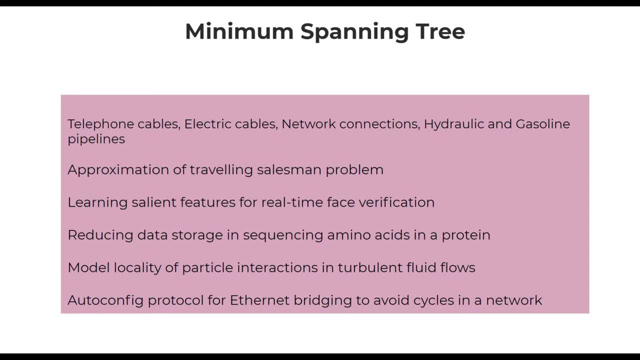 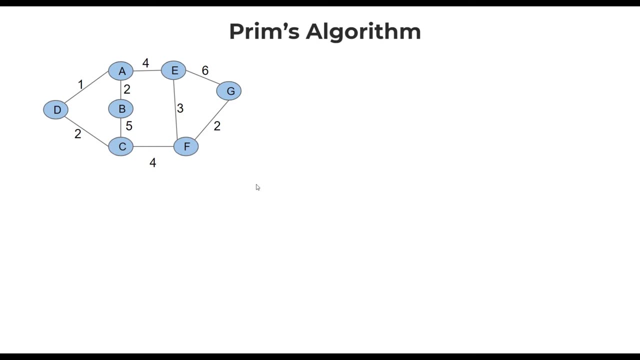 there are several other applications as well, like approximation of traveling salesman problem, real-time phase verification, amino acid sequencing, particle interaction, ethernet bridging protocols. let's take this graph and try to construct a minimum spanning tree for this graph by following a greedy technique. to begin with, we can pick any vertex. i am picking a. consider this a to be. 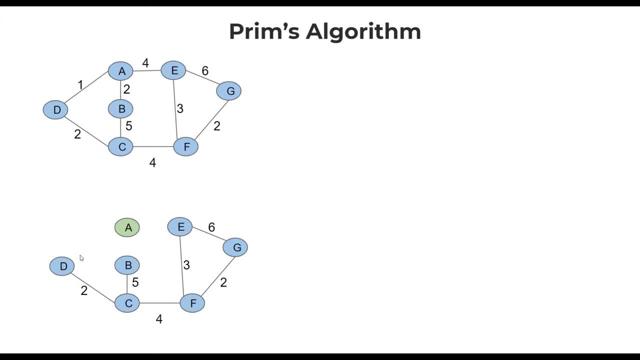 disconnected from the rest of the graph. now our intention will be to somehow connect a to any of these three vertices. the edge weights are one, two and four. since we are following a greedy technique here, we will obviously choose this edge, as this has the minimum weight. now, a and d are part of the spanning. 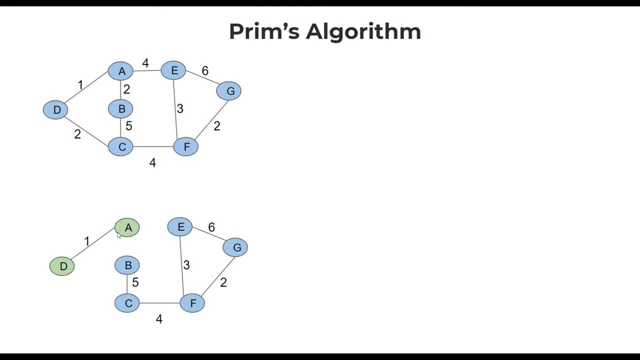 tree that we are constructing. now we need to connect this part to the rest of the graph. we have quite a few options here. a could be connected to e, a could be connected to b or d could be connected to c. both these edges have the same weight, so we can pick any of them. 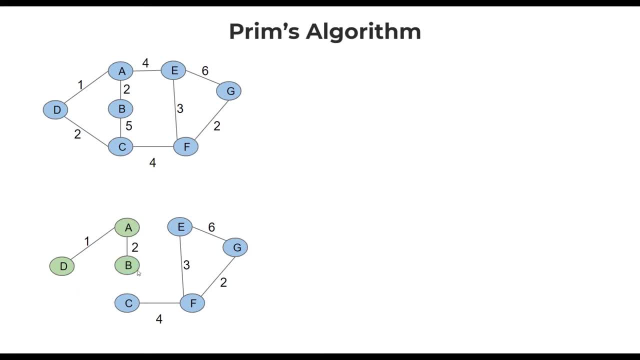 let's pick this one, a, b. now, on attempting to connect this with the rest of the graph, we again have three options, and we would prefer the one with the minimum weight here. d, c. now to connect this with the rest of the graph, we have two options and both have equal weights of. 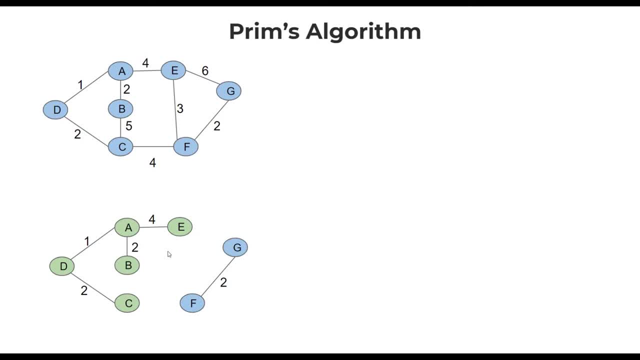 four. let's pick this one, a, e- now to connect this path with the rest of the graph. we have three options. we always choose the minimum edge, so let's take three here. now to connect this with the node g. we have two options and we would prefer this one because it. 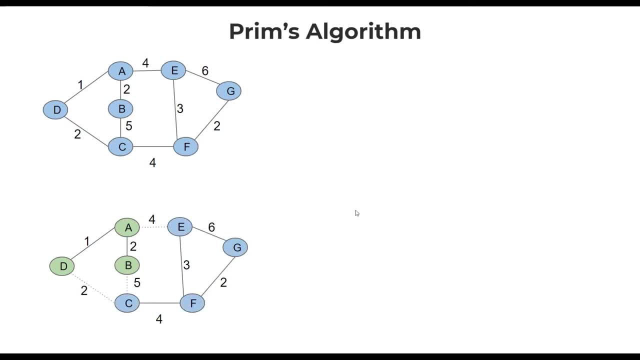 has the weight of two. as we add more and more vertices to the spanning tree that we are constructing, we ensure that during each addition we select the least value. certain greedy algorithms may not give the optimum results all the time, but prim's algorithm always promises a minimum. 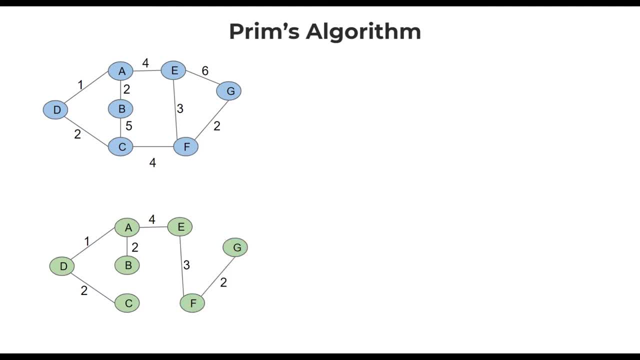 spanning tree by contradiction. if we assume that prim's algorithm is not giving us a minimum spanning tree, it means that in the process we have picked the wrong edge. we did not pick the minimum value at some point of time, which will never happen if we implemented the algorithm. 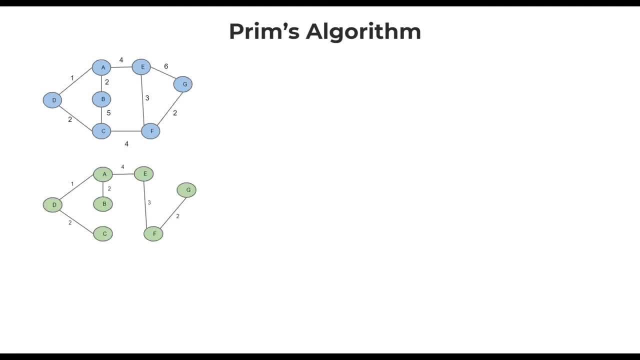 correctly. all right, now, instead of giving the names as abc, let's change it to 0, 1, 2, 3, 4, 5 and 6. let's try to write the pseudocode for this. say: we are given, with the, the, the, the matrix of the graph. this visual is just for our imagination. we only have this matrix as 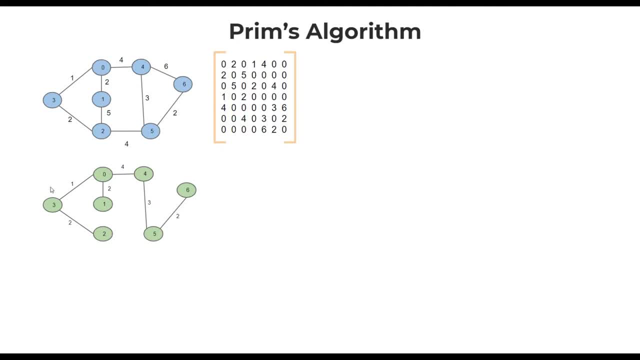 the input. how are we going to express this spanning tree? as a result, we can simply have an array, a parent array, which could tell us what is the parent for each of the vertex. see here, in this spanning tree that we have constricted. if you take the vertex 1, 0 is the 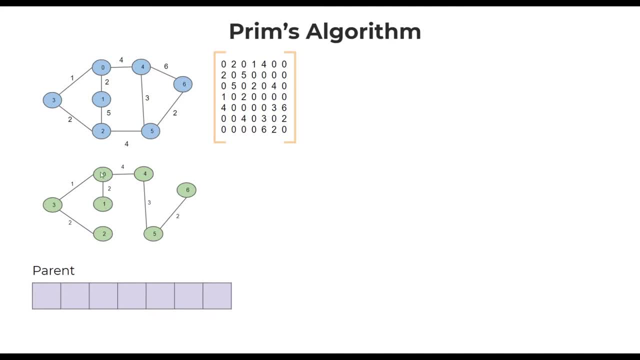 parent of 1. similarly, 0 is the parent of 3 and 0 is the parent of 4 as well. so if we have such information in an array and also this adjacency matrix, we can easily constrict this spanning tree. so our code should be able to give us a result like this. we are going to start with some vertex. 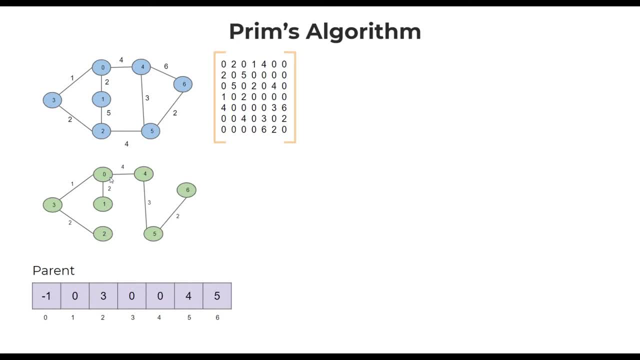 and then we are going to add more vertices to our spanning tree, right? so we obviously need some kind of boolean array which could tell us what are all the vertices that have already been added to the spanning tree and what are all the vertices that are yet to be added to the spanning tree. so let's. 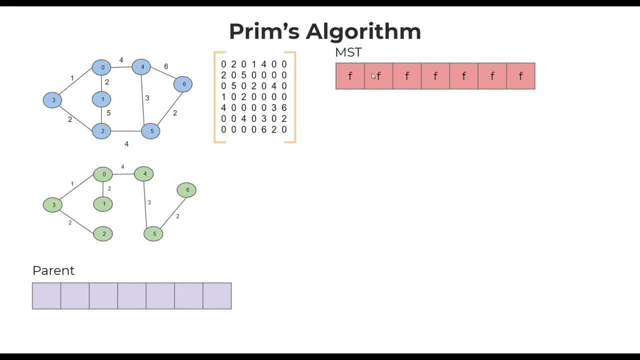 have an array for that and we can easily construct this spanning tree. so we can easily construct this spanning tree. we can initialize it as all false in the beginning. we can pick zeroth vertex as the first vertex in the boolean array. we can mark the zeroth vertex as true, as it is now part of the. 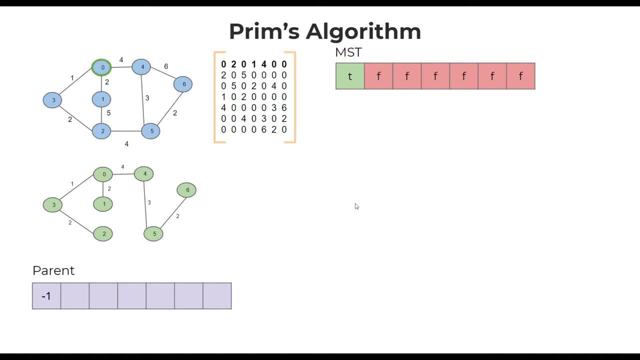 spanning tree. moreover, the starting vertex cannot have a parent, so we are assuming that the parent of the starting vertex is minus one. now we can go to this zeroth row of the adjacency matrix. it will tell us all the connections from zero. so we have three edges, with the edge weights two. 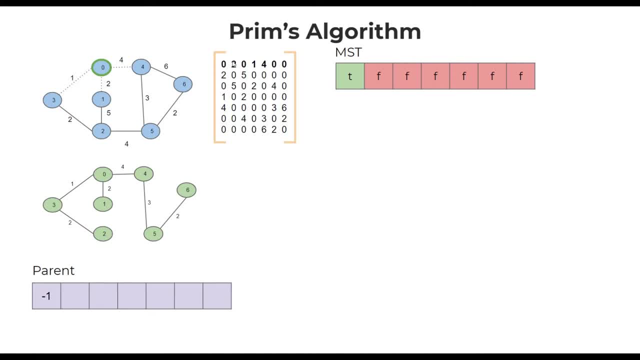 one and four. we would like to pick the minimum value here, which is one, and it belongs to the third vertex. the column number is three here, so we include this three also in our spanning tree. we can mark true here for the third vertex, and also now the parent of three is zero. we have included this vertex three. 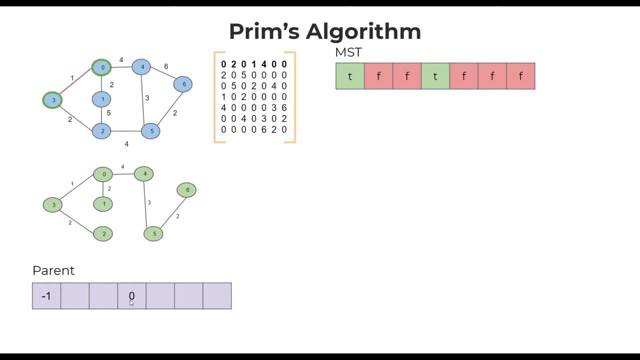 by connecting it to zero, right? so here the parent of the third vertex is zero. now we have two vertices in our spanning tree. we have to loop through both of them and pick the minimum value, but also ensure not to pick the value that we have already picked. 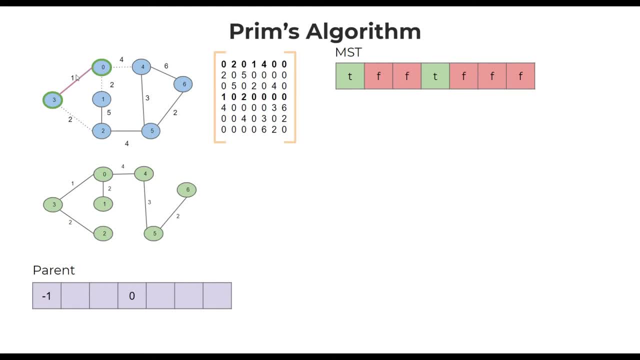 see here, one has already been picked. we have to pick the next minimum value. as we add more and more vertices to the spanning tree, this process is going to get difficult right to pick the minimum value, so we kind of need to have a workaround here to make the process simple and quicker. 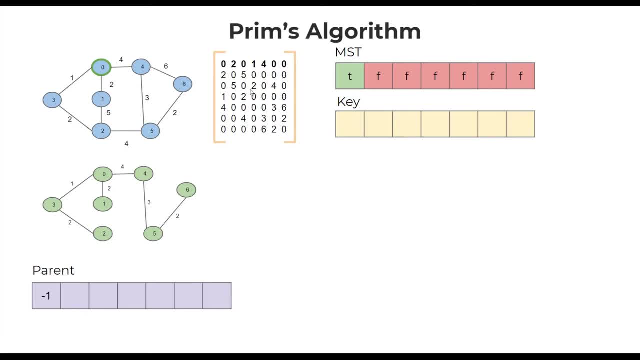 we can have an array in which we are storing the minimum key values for each of the vertices. we can initialize them in order to construct a new key value for each of the vertices. we can initially the values to some maximum integer value for all the vertices except for the first one. we can assign. 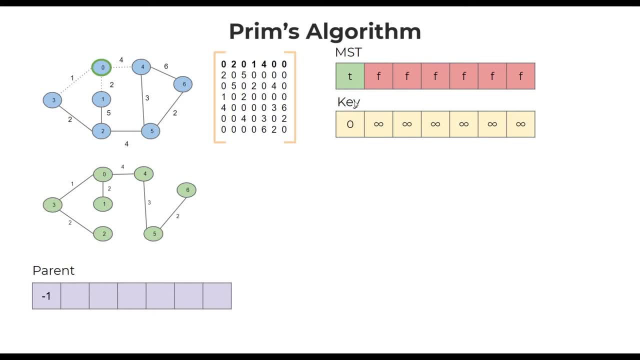 a zero for the vertex that we are going to pick first, because we are always going to pick the vertex from this key array, which has the minimum value. so initially we pick this zeroth vertex. since zero is our first vertex, we go to the zeroth row of this matrix and loop through this row, while 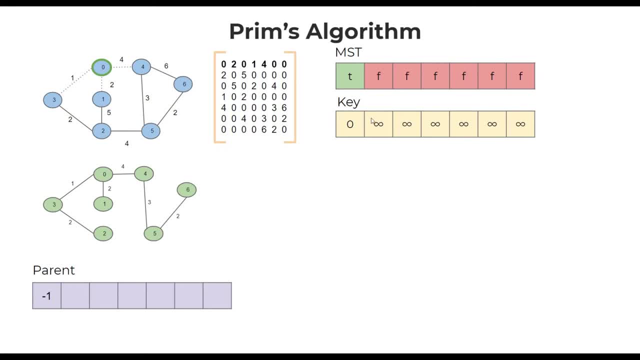 looping through this row itself, we can update the corresponding key values to one and four. if we update like this, it will be very easy for us to pick the next minimum value. see here: zero we have already picked. you can just cross check with the boolean array. now. the next minimum value is one. 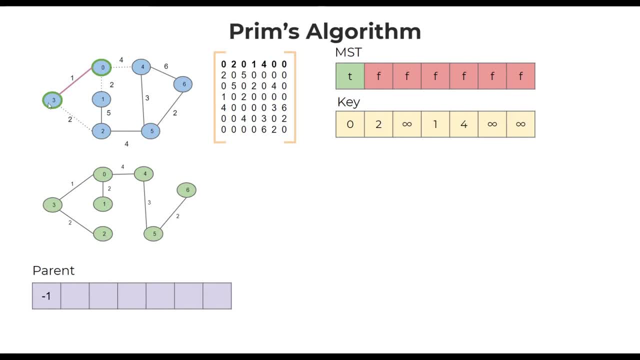 which corresponds to third vertex, so we can include that vertex to our spanning tree. now what we can basically do is, while looping through each of the row, we can just look up this table. if it already has a minimum value, we can ignore. but if we have a better value now, while looping through, 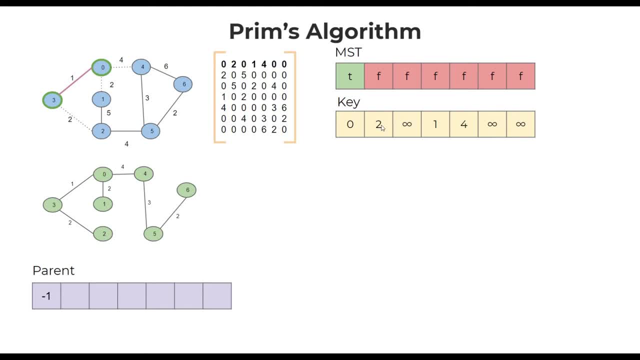 the row. we can update that better value to the key array so that we always pick the minimum value. we can start with the zoodo code. you can understand better as we progress. we can initialize three different arrays: for parent, minimum, spanning, tree, boolean array and the key array. we can first 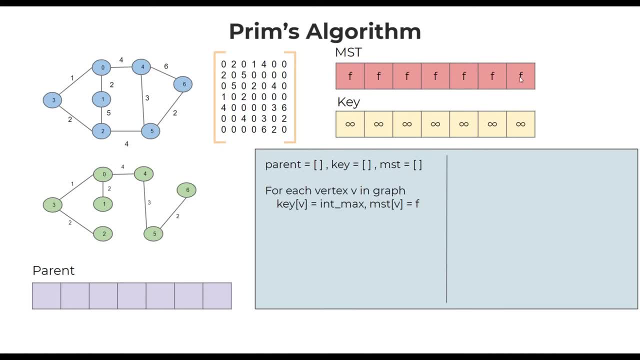 initialize the boolean array to all false and the key array can be initialized to all infinity. that is some maximum value for integer. we can now change the key of the zeroth vertex to zero, so that this get picked first and then the parent of the zeroth vertex will be minus one. 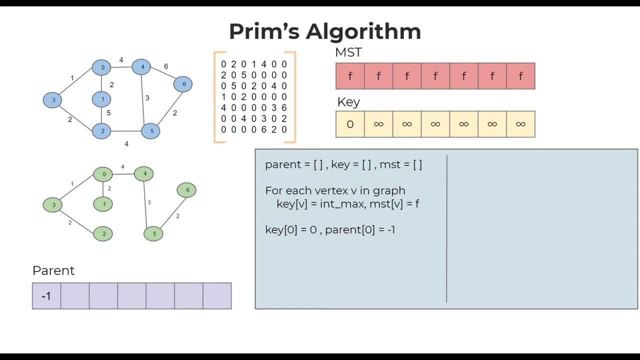 now our first step is to pick a vertex. right, we always pick the minimum value from this key array. so for each vertex we present in the graph, we just loop through this key array and pick the minimum value, but also make sure that that minimum value has not been picked already. you can find it by: 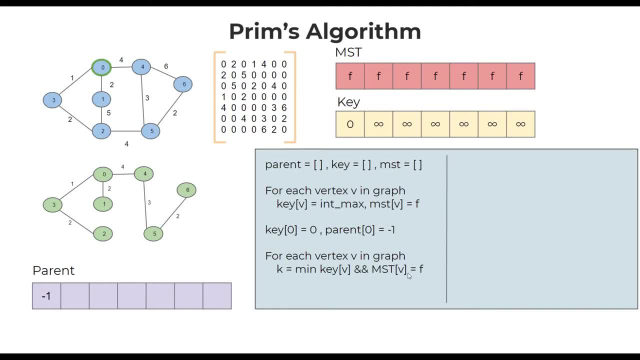 just looking up the boolean table. we pick that vertex only if the value is false in the boolean table, only then it has not already been included in the tree. if it becomes true, then that vertex has already been included in the spanning tree. so we should not pick that minimum value we have. 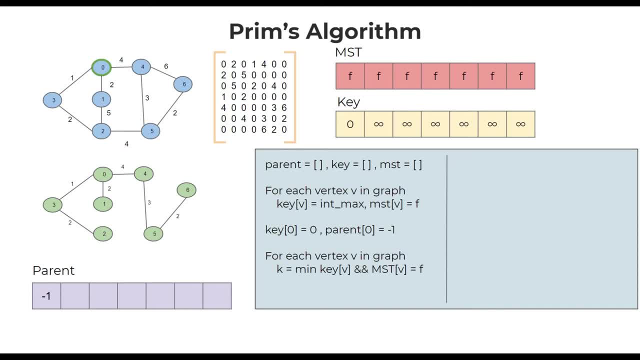 picked a vertex, k. now this k has to be included in our spanning tree, right? so we have to pick the minimum value, so we can just mark the msd of the kth vertex as true. now we have to loop through this row of the adjacency matrix, right? so for each vertex present in the graph, if the value is less, 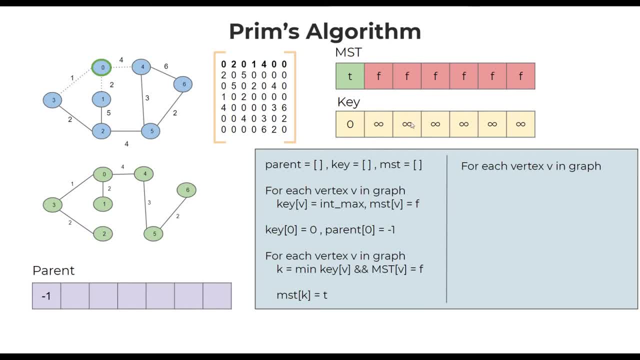 than the value present in the key table. we have to update the key table, right, so we just have to compare each of these values to the value already present in the key table. since we are dealing with an adjacency matrix here, there will be lot of zeros as well, and we should ignore the zeros. so 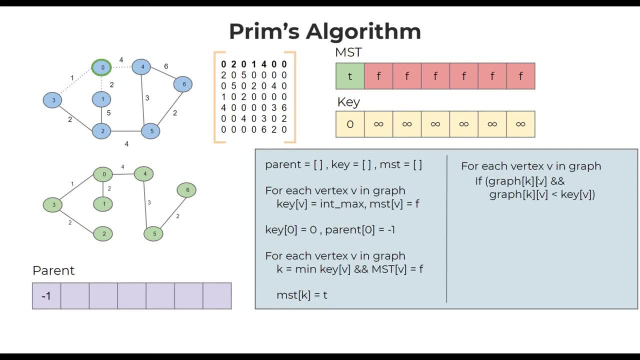 only if the value is greater than zero and if it is less than the key value already present in the key table, we have to update the key value present in the key table. so here, in this case on comparing, we can update these three values- two, one and four- to the key table. for all these three vertices, see: 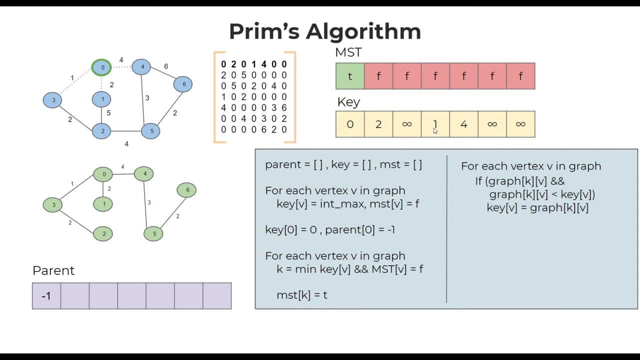 here. this is the first vertex, this is vertex number three and this is vertex number four. right for all these three vertices, zero is the parent, so we can mark the parent as well. this is definitely not the final value of the parent table, if we are able to find a better. 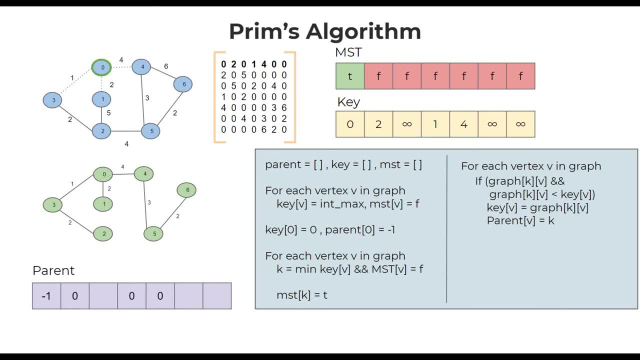 edge, then we will update the key value table and also the parent. we do all these steps inside the loop, so now we go back to this step to find the next minimum value. right, the next minimum value is one, because zero has already been marked as true, so we have to pick this value, one which? 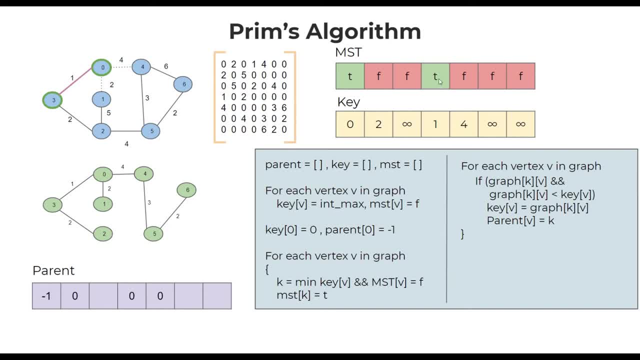 corresponds to the third vertex. so we are marking the third vertex as a part of spanning tree. just make this as true in the boolean table. now we need to loop through the third row of the matrix. now we start comparing the value one by one. here we have a one. 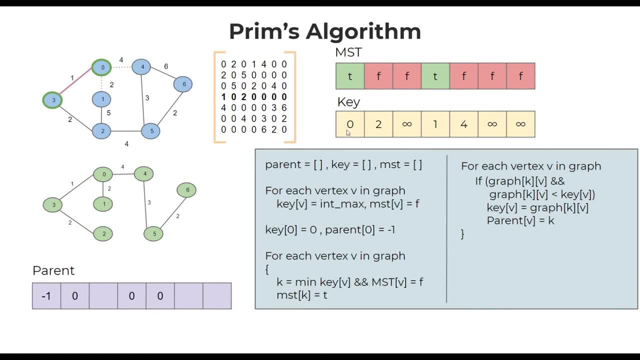 and a zero. we don't have to update. moreover, this first one has already been included in the tree, right? so we don't even have to compare for the key values that have already been included in the spanning tree. so we can add one more check to save some time. we can compare only if those vertices. 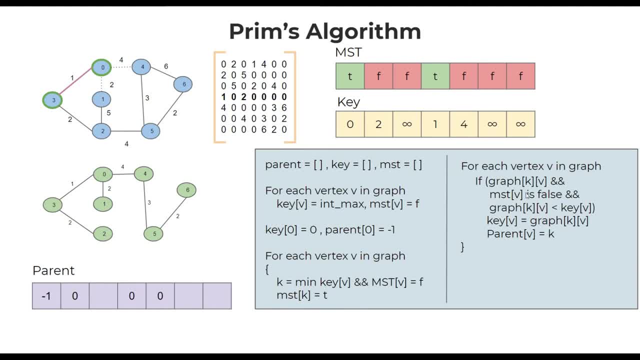 are not the same. so we can add one more check to save some time. we can compare only if those vertices are not been already part of the spanning tree. so if mst of v is false, only then we update the key values. if it is already true, we don't have to update now. this value is 2 here, but the corresponding. 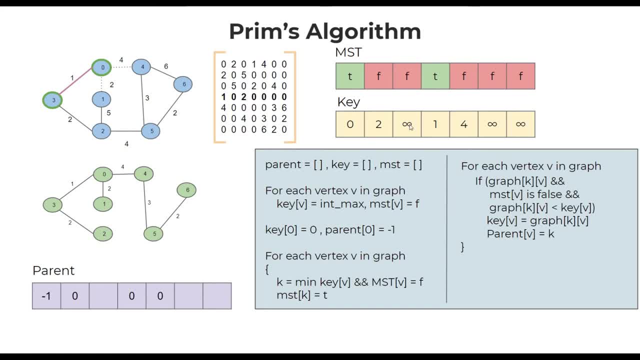 value in the key table is infinity. on comparing, we are now getting a smaller value and we can update that value in the key table. the parent of this node would be 3, because we are in the third row. now we are looking up the adjacency matrix for this third vertex, so this vertex is now the parent. 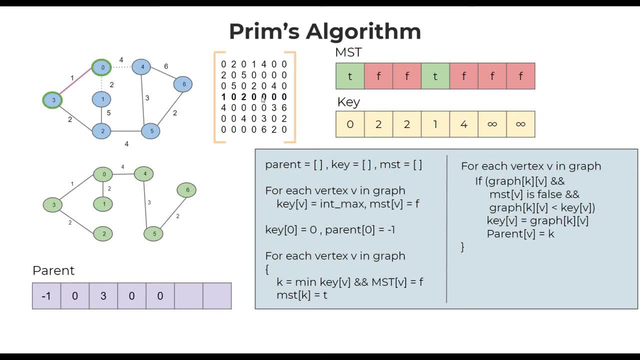 for all these connections. so we can update a 3 here in the parent array as well. going back to the top of the loop, we have to pick the next minimum value. we have two twos here. as the next minimum value, we obviously go with the first available option. we pick this two. this corresponds to the 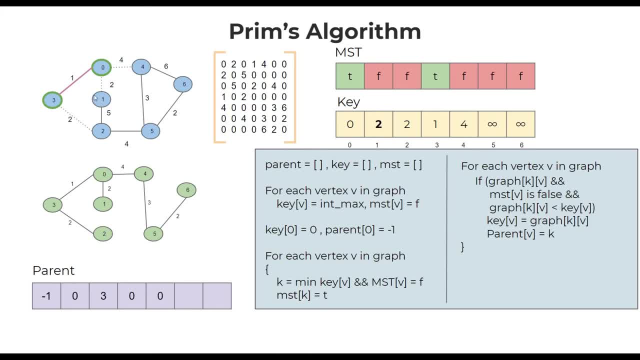 first vertex of the graph. so we include this first vertex to our spanning tree. just mark the corresponding boolean value as true. now, on looping through this first two vertices, we can update the row of the matrix. we have two values, 2 and 5. we don't have to update this too, because the zeroth 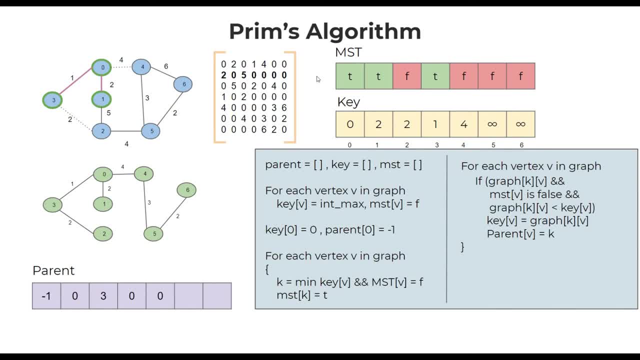 vertex is already part of spanning tree. so take this value 5. when we compare it with the corresponding value present in the key table, we see that it already has a smaller value. right, there is no point in updating a bigger value to the key table. we always want minimum values in the key table. 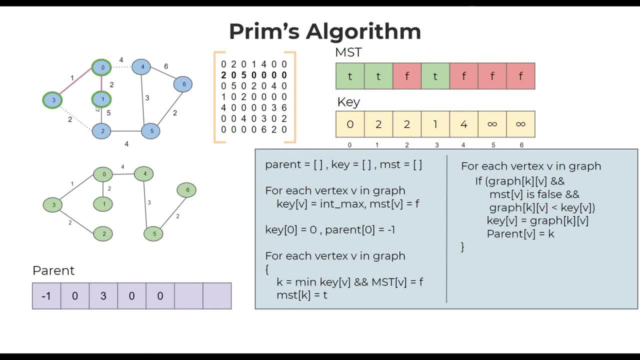 so we just ignore this edge 5. we can just remove it out of picture. we don't need it anymore because we have a better option. that is this vertex here. we have already updated that there is a connection from parent 3 with an edge weight of 2, so we are now ignoring this connection, okay. 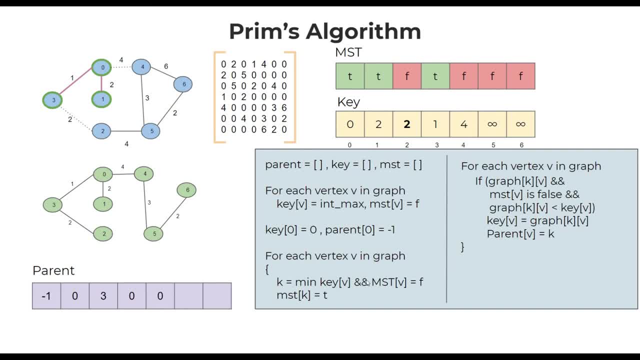 now again going to top of the loop and picking the next minimum value, this 2. here it corresponds to vertex number 2, this vertex. so we are including that as part of spanning tree so we can mark this value as true here. now we have a better option, that is this vertex. here we have already updated. 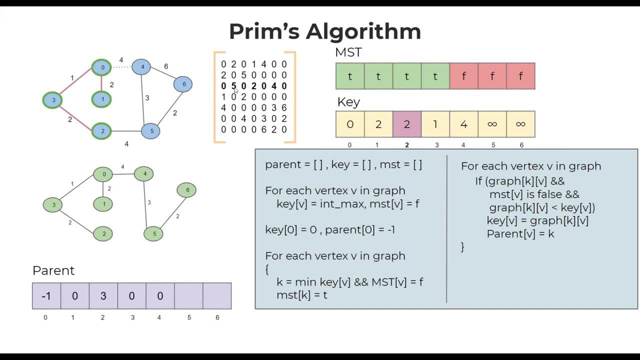 looping through this row. we have three values: five, two and four. we see that this five and two, the corresponding vertices, have already been added to the spanning tree, so there is no use of comparing these two values. we just need this four. if we compare the corresponding value in the key table, we have an infinity here, so this has to be updated. we update that. 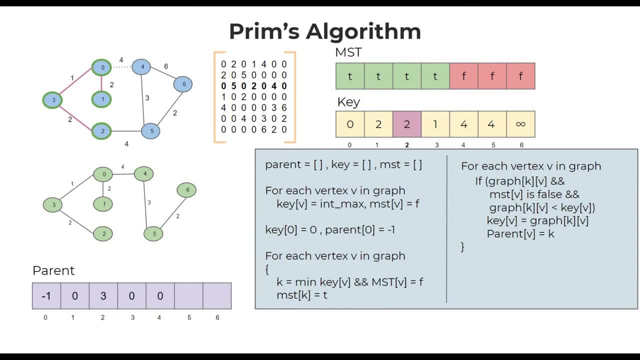 as four and the corresponding parent should also be updated. we are in row number two, right, so here the k value is two and that is the parent for this vertex. now, taking the next minimum value from the key table, it is four. it corresponds to the fourth vertex, so include: 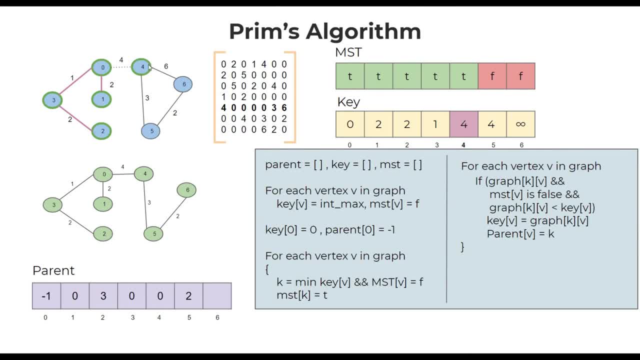 the fourth vertex as part of the minimum spanning tree, mark the corresponding value as true in the boolean array. on looping through the fourth row of the adjacency matrix, this is the fourth row. i am taking this one as the 0th row, so this is the fourth row. on looping. 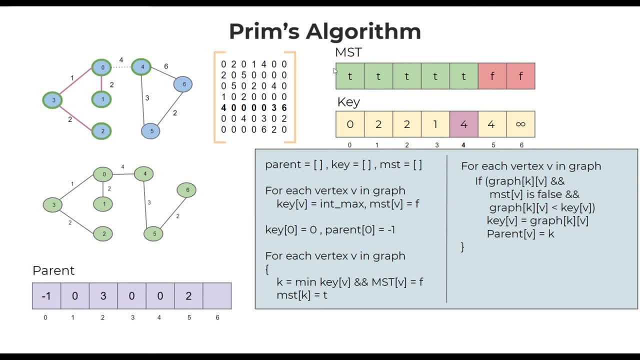 through this, The value 4 here is useless because the corresponding vertex has already been added to the spanning tree. Now take this number 3.. The corresponding value in the key table is 4.. It means that this 5th vertex right here has some other connection with an edge weight of 4.. 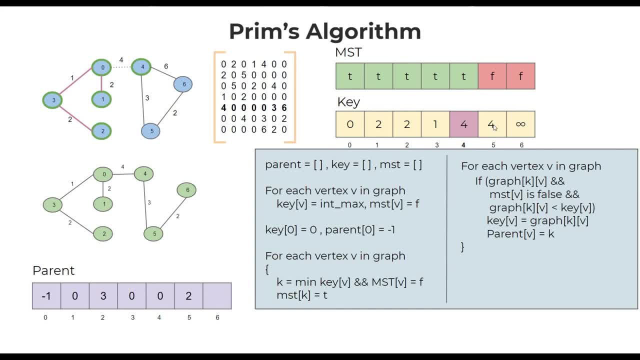 You can exactly know to which node it is connected with the help of the parent table. It is actually connected to vertex number 2 with an edge weight of 4.. See 5 right here is actually connected to vertex number 2 with an edge weight of 4.. 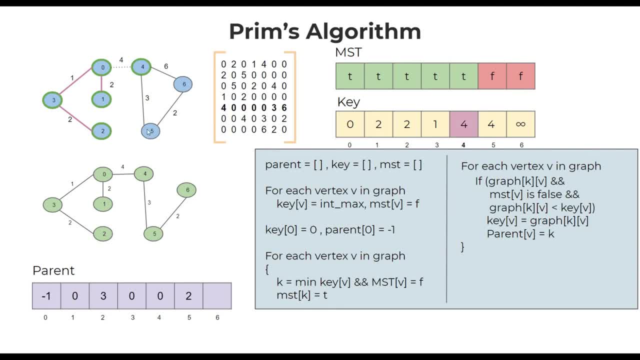 But now we are finding a better option with an edge weight of 3 here, So this 3 has to be updated instead of 4.. We have found a lesser key value now, So just update this as 3, and the corresponding parent should also be updated. 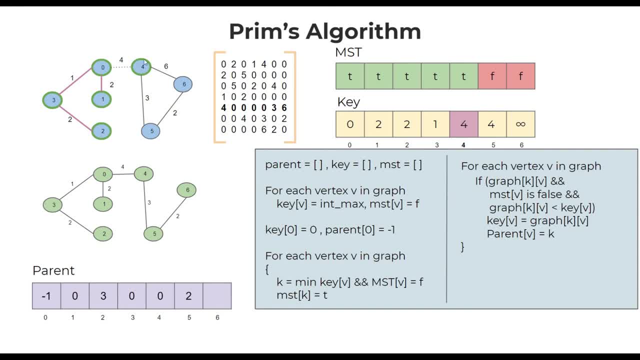 The corresponding parent is vertex 4, because we are in this 4th row, So here also we update the corresponding parent. And also there is 1.. One more value: 6. It is already infinity in the table, So this also has to be updated. 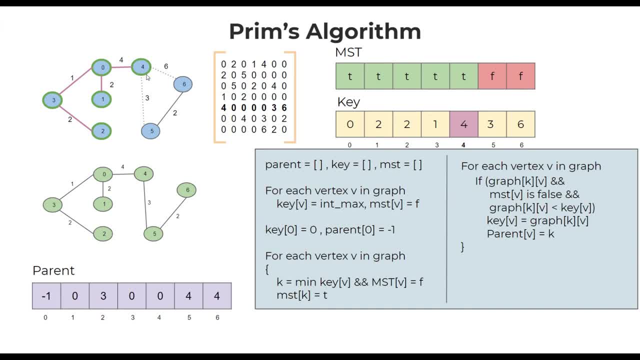 Let's make it as 6 and the corresponding parent as 4.. Because now k value is 4.. Now picking the next minimum value: it should be this one, The 5th vertex, because the value was 3.. So we mark the corresponding Boolean value as true and include the 5th vertex also to our spanning tree. 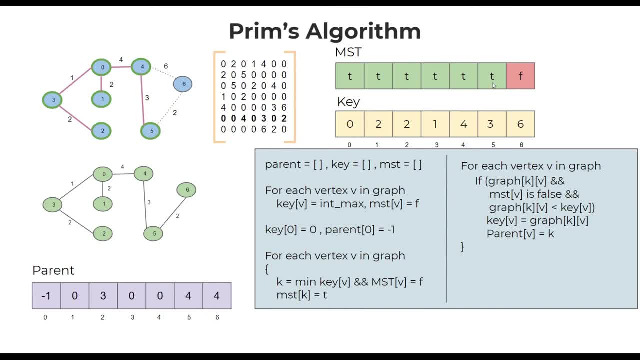 All these values are true. We just have to compare this last value. This is 2.. But the key value that is already present is 6.. We now have a better value, So this has to be updated. So make this 6 as 2..